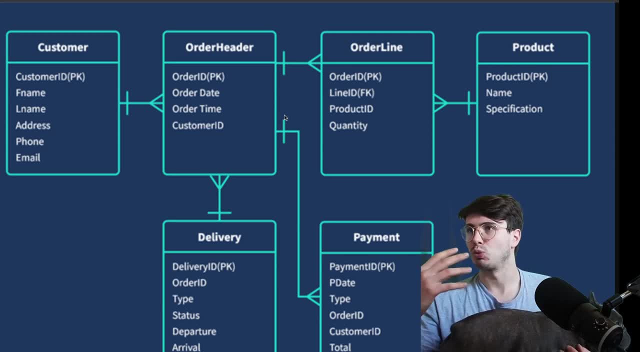 give you an example of you know, hey, how does this work, And you know what is the initial type of data modeling Before that. so, just high level data modeling is, you know, really it's the art and kind of the science of framing data in a manner that makes sense, but it also can be easily. 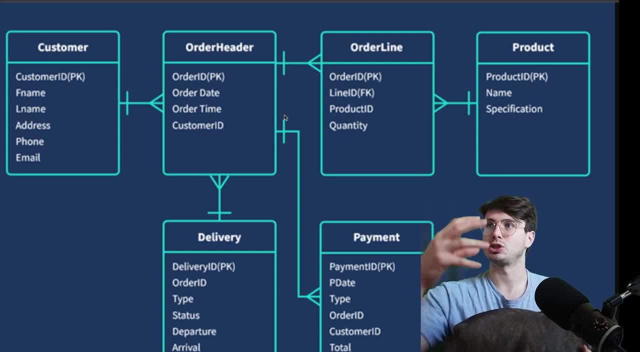 manipulated and analyzed. So it's not just for you know, making this human readable, it's also making sure that your queries are really efficient so that you can save money on the compute needed to actually run those queries to access information you need when you're doing, you know, large scale. 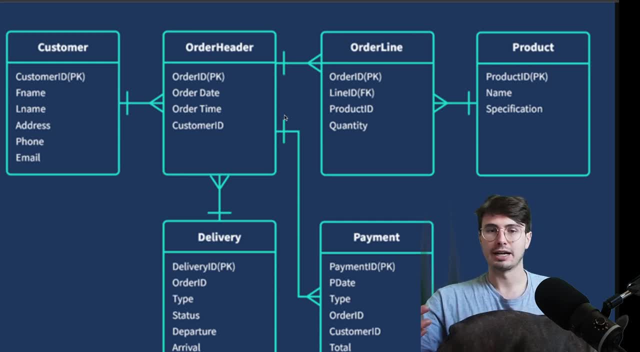 data modeling, And so you know the cost of you know going through millions and millions of lines of data can become quite significant. So this provides you know foundation, for by having cleanly ordered data that's easily queryable you can really provide solid foundation for many. 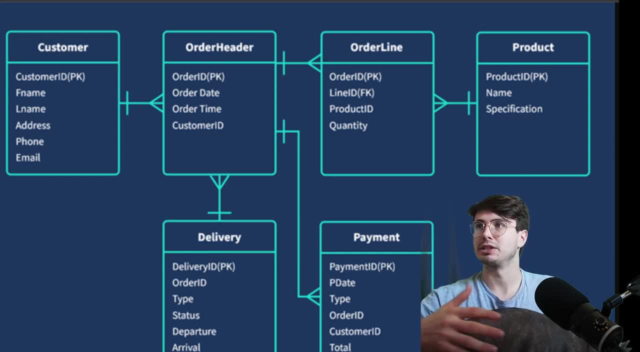 different applications, like you know: database design, machine learning algorithms, bringing your data directly from here, you know, into some kind of analytics platform. it just makes everything you're doing on top of the data much easier if you have a very clean and structured data model, And so you can. 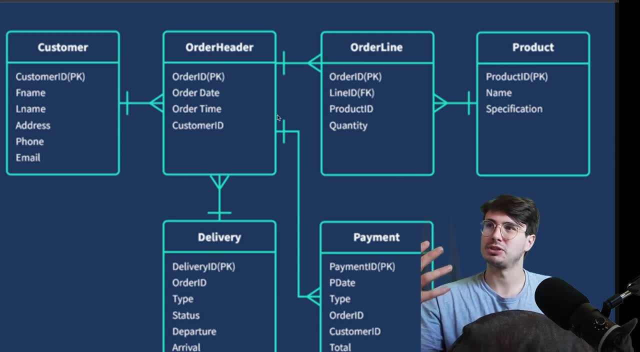 kind of see here. within this it is really a conceptual representation of data objects. So you know, obviously this is, you know these are gonna be different tables within a database, But at a high level you're going to want to, you know, kind of diagram it out to make sure, hey, do these relationships between 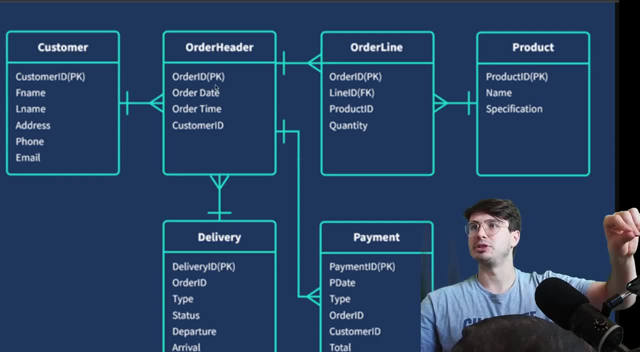 you know payments being linked to the order object makes sense And is that like, logically, where I'm typically going to get the payment information from by querying that order header? Or maybe it should be under customer, because you know I want to look at all the customers payment information And so that's. 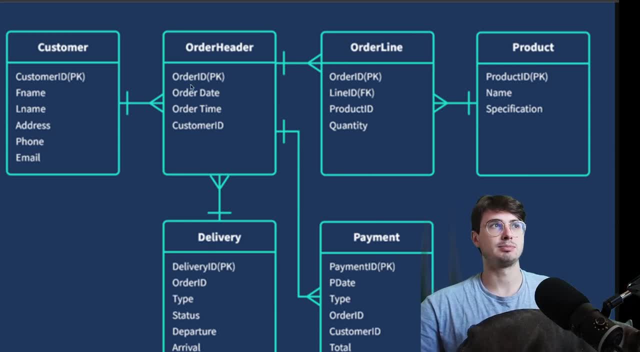 kind of a choice You know this user has made, where they have payments being linked directly to order header rather than by customer, but there is a customer ID within the payment object. And so you're looking at you're not only the representation of data objects, the relationships between them, the rules governing these relationships. So you 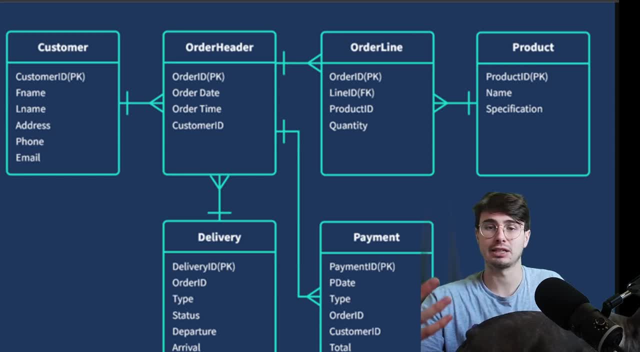 know you don't the rule that, hey, maybe in this you never put payment information in the customer object And it's really just a blueprint for as you build and ingest data, guiding the structure of the data in kind of a systematic and standardized way. So just to kind of walk you through what this data model is here so that I can. 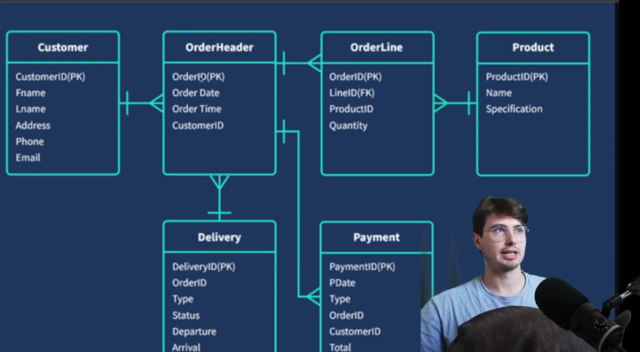 talk about maybe some of the example applications and why it's useful. So here we have, you know, the base object or maybe your you know order header. So every time you know customer makes an order, there's an order header which has an. 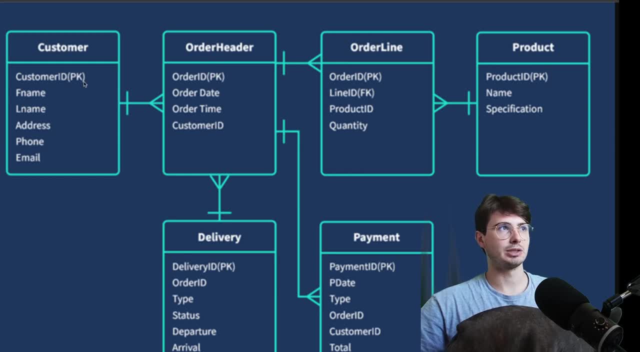 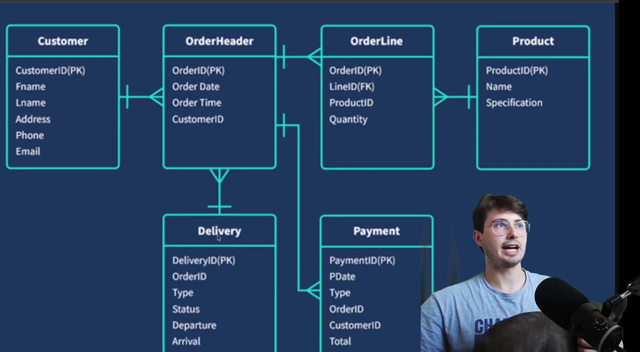 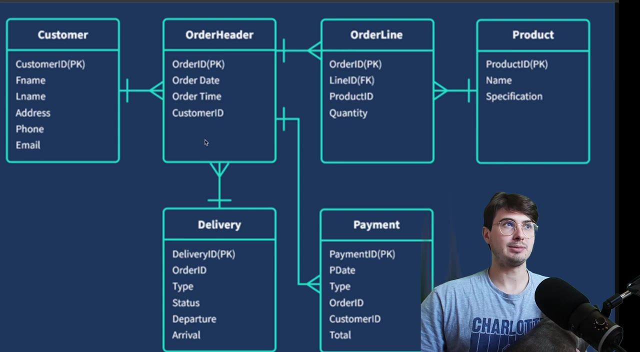 order ID, order date, order time. customer ID which links to the customer and all the information about them that they purchase this for. It also has a linkage to the delivery ID, So it's actually not the delivery ID. references the order ID, So already doesn't reference the delivery ID Because 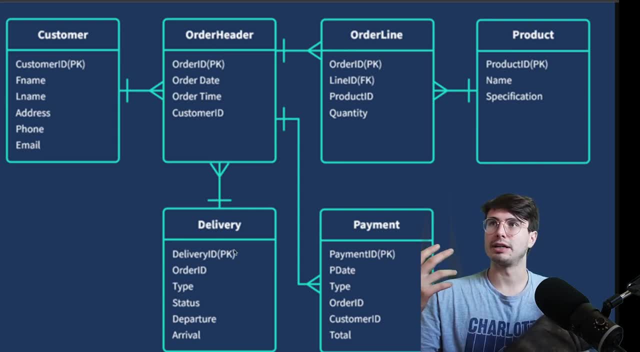 typically, if we're looking at delivery information, we're not or we're just going to do already from there. But if we're looking at the order header information, we're not going to typically need the delivery information because maybe we're just 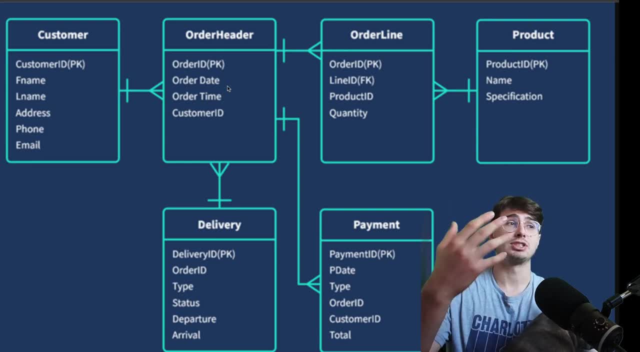 looking at the payment And this is one of those decisions that, hey, you know I didn't make it, But someone made this decision to say: you know, we don't actually deliver ID and order header to save space on storing that twice Because some of 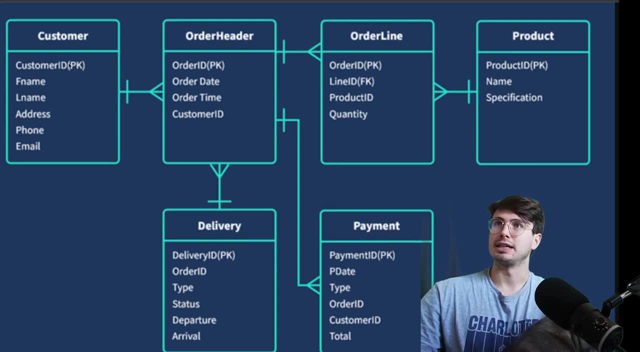 these fields like customer ID, here under payment and in here you have PK. So within each table you'll have a primary key And what that is is the totally unique identifier for each object. So there can no be no duplicate customer IDs within this table And the customer. the primary key here is how. 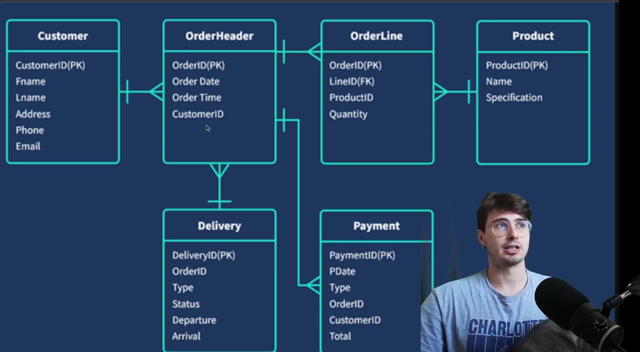 you can reference this tables. So here, customer ID, referencing customer here. But this is basically your single source of truth that, hey, every customer is going to have a unique ID. every 99% is going to have a unique ID there, Remember primary key: every order ID is going to be unique And 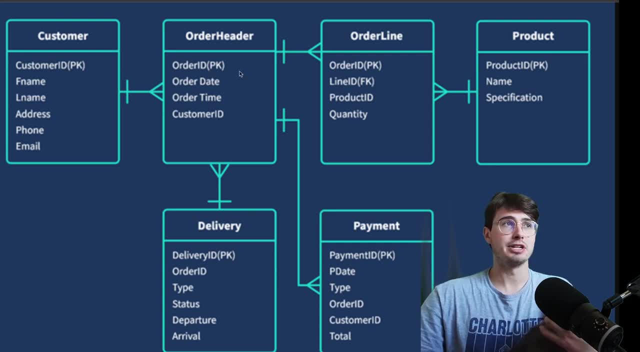 maybe you know two people made the same order on the same time, But they're going to be distinguished by their different order IDs. Even if a customer made an order twice- you know, maybe they fat fingered click it twice- there's still going to have two separate. 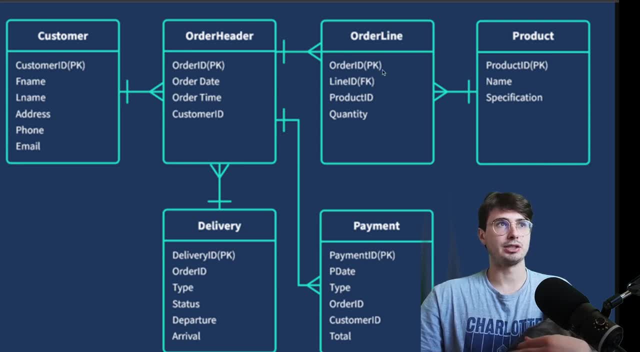 old parties to differentiate them. And then we here under order line, you have primary key, line ID, which is a foreign key. So this means it's matched his a primary or table. So this means that this key isn't actually present in all of this information. So this is: 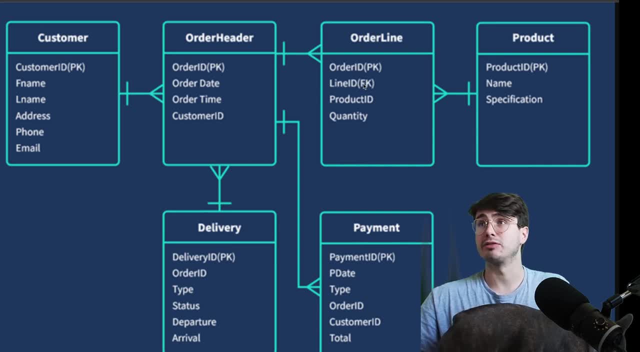 being pulled in from a line information. you know, maybe that's the head database, where it actually just stores all the different orders separately, And so that's, if you need to bring information from a separate database, you can use foreign keys that will match another unique identifier. 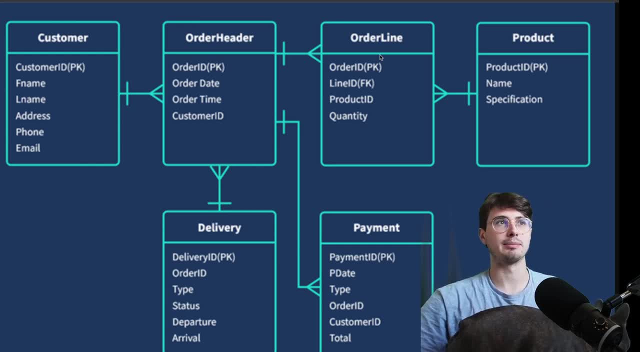 So the line ID will have to be unique in another table that this is pulling from. Then over here you have the product ID with the product unique identifier name specification, because you know that's all the information you need about a product because many people are gonna be buying. 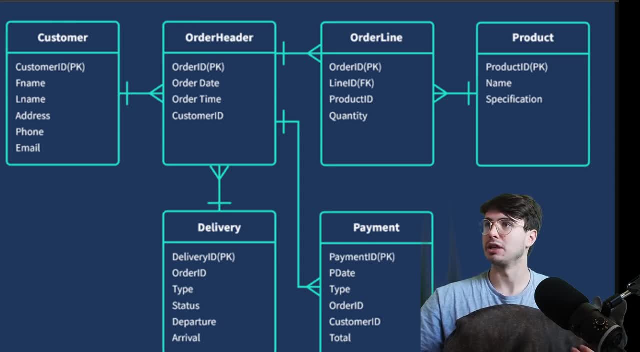 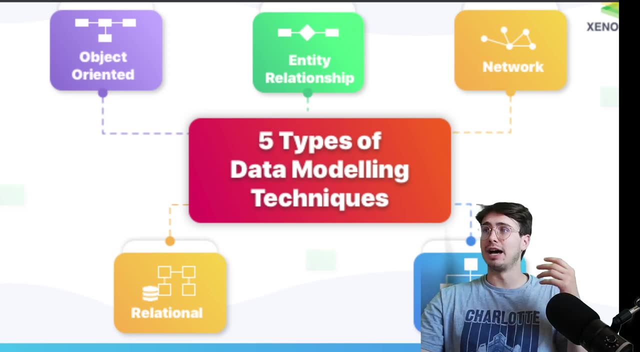 it. many people are gonna be referencing it, So you don't need a lot of unique information there other than each product is obviously its own type And so that was actually only one type of data model. You also, that was the relational model, So with the relational model it is rep. 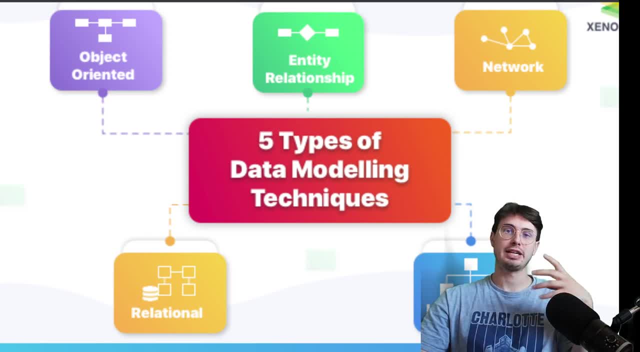 you know, you have concept of relations which are represented by different tables, And so tables are used to store data, Establish the relationships between those different data elements, So by primary key referencing each other, and it's widely used because it's relatively simple to set up. It has 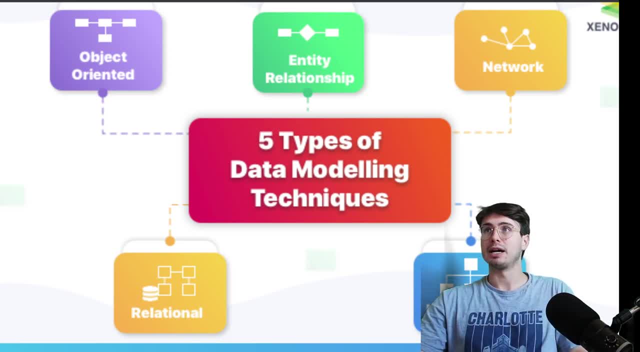 really powerful query abilities as well. You also have object oriented data models, And so object oriented data models combine data and the operations that can be formed on data, like extracting into a model, And so this is really useful in applications where you need you know. 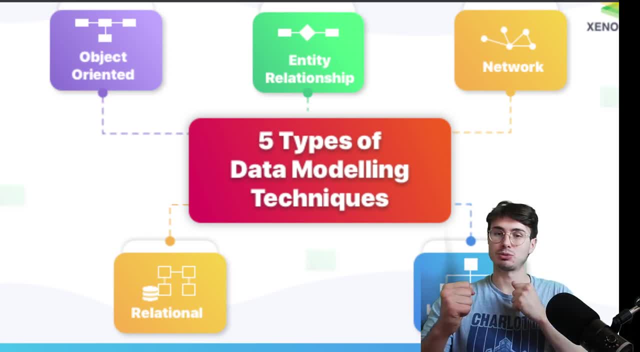 real world representation of your data, with complex relationships and operations Where you have, you know, maybe not a large amount of objects, but each of those objects has to store a lot of different state changes. You know, maybe it represents maybe an AI model that has you. 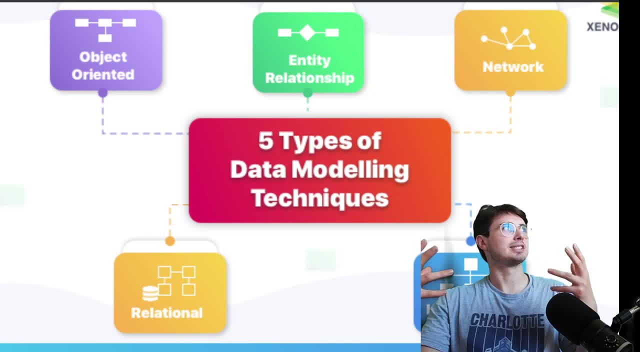 know all actually, no, that wouldn't make any sense, Sorry, maybe it represents, like the ingestion of a or the robotics of a car factory robot and all the tons of crazy information about all the different operations it's performing. You also have network data models, And so these kind of 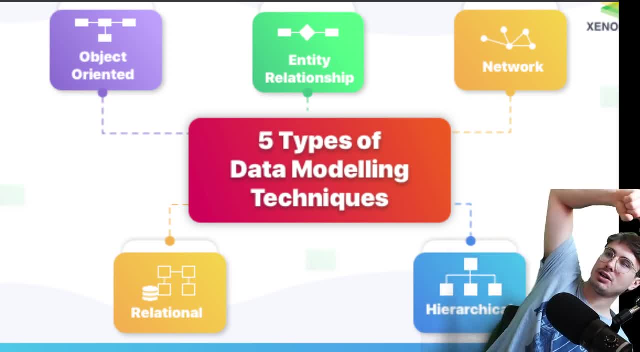 are an extension of this: hierarchical data models, which are basically just a tree like structures. you can see here kind of looks like a tree: Each record has a single parent and set zero or several children, And this is kind of an earlier database system where you didn't really have a lot of data. 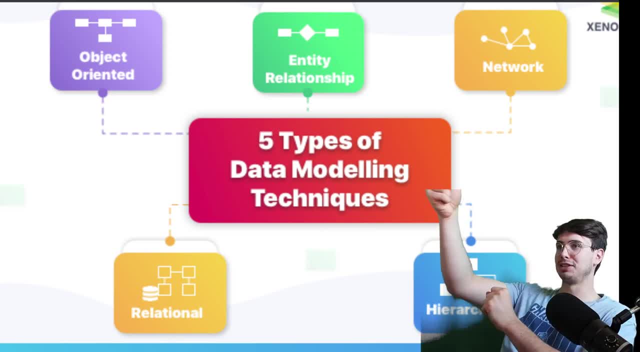 So you'd have like, hey, this company has this many users, and then you kind of have, you know, like almost like a leadership chart of each manager has several people under it, but it really has limitations when you want to represent many, many relationships. you know maybe the relationship between using that kind of worker. 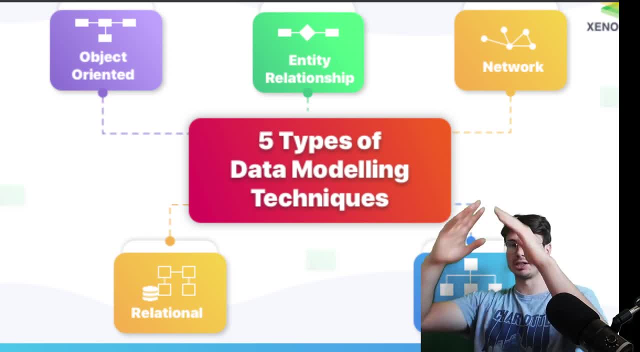 analogy like relationships between coworkers. you couldn't do that. it'd have to go through their manager, And so that's where you had the network model come in, where you have multiple parent records for each child So you can have you know one child is linked to many different. 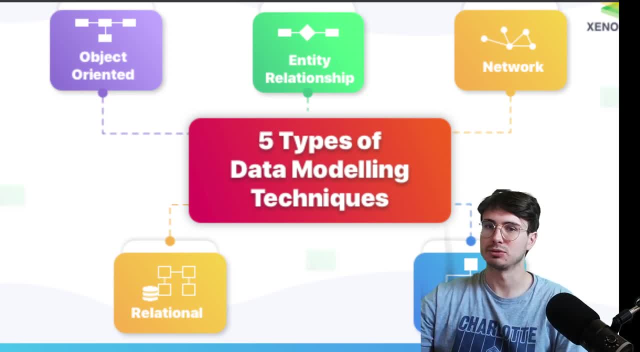 parents And that kind of allows you to represent more complex relationships and you know kind of work around the limitations of the hierarchical data model, but wouldn't say it's super popular these days. Then there's also the entity relationship model, which is widely used in database design And that's where you have entities attributes. 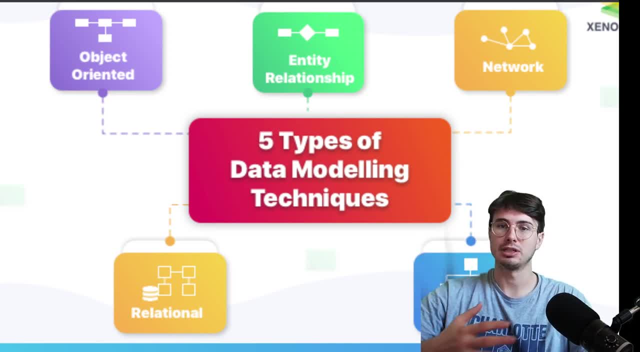 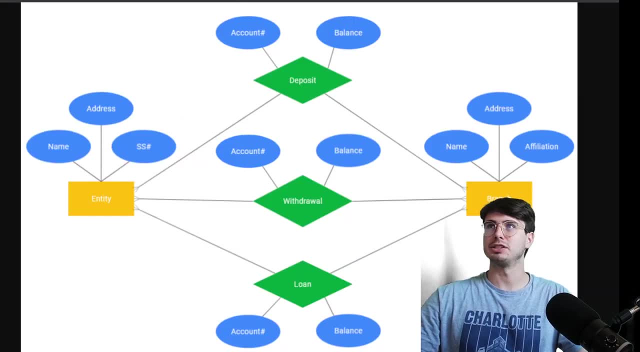 relationships amongst entities, helping you to kind of have a really clear logical view of the data, So that where it is, you know, almost just like a mapping of relationships between things. So here you have an address, name, affiliation for, like a bank branch, you have withdrawals account number. 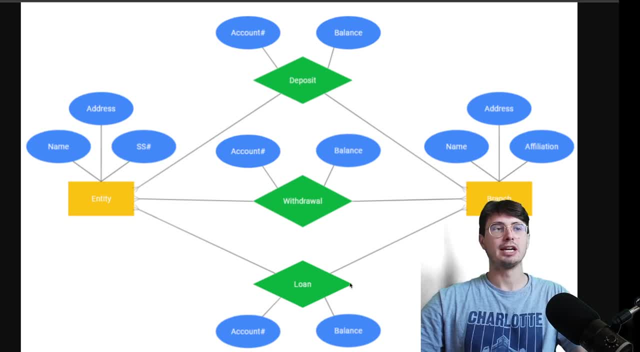 balance, deposits kind of, which also inherits from account balance, And this is, you know, great for when just have a lot of different things that all relate to each other. So maybe not or not a lot, but a relatively small amount of things that have really defined relationships that you 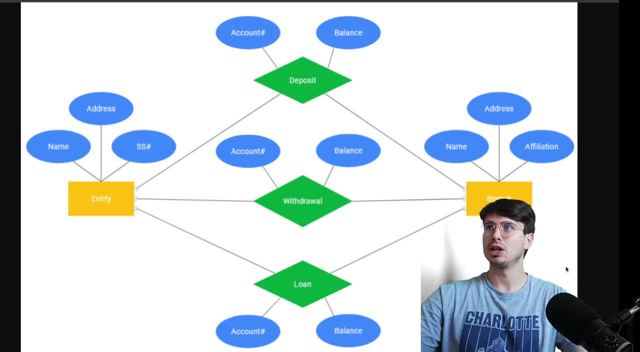 are you know know are going to happen. So you're always gonna have to go to deposit or draw from a bank. it's always gonna be a you know user that does that, And just having that very clear model to understand how your data is flowing makes it easy to process collect. 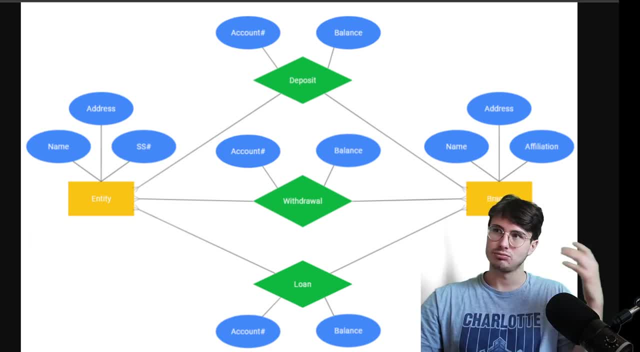 and then you know, query down the road. So really, you know, just easy to look at when you compare it to maybe something like that, A relational data model, where it does take, you know, a little bit of kind of thought conceptualization to really get them, And so 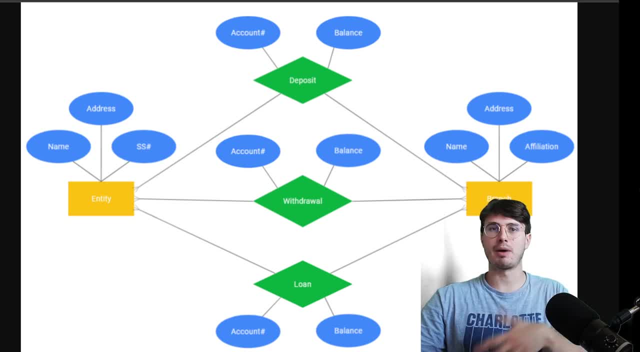 those are kind of like all of the different you know, actual data models. you know in terms of implanting. there's also things like conceptual, logic, logical data models that are just high level representations of your data. But that's not. 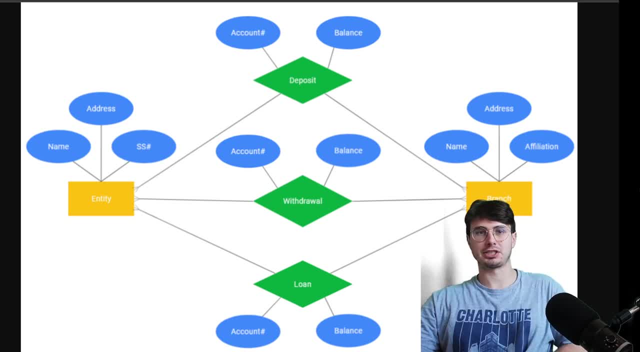 really what you'll be using in practice if you're implementing data modeling, unless you're just visualizing it to an external stakeholder. So some of the applications of data modeling kind of moving on now, And so now to kind of bring it all together, you know how is data modeling used. 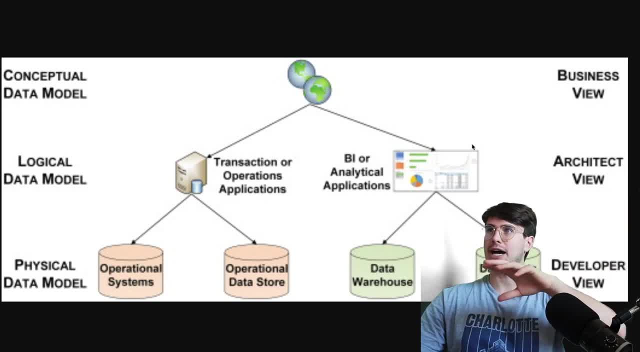 in the real world. So there's a conceptual data model right at the top. that's really just the business view of understanding. you know how. you know how you're going to implement data modeling and how data is flowing through your business, how it's going from. you know your front end. 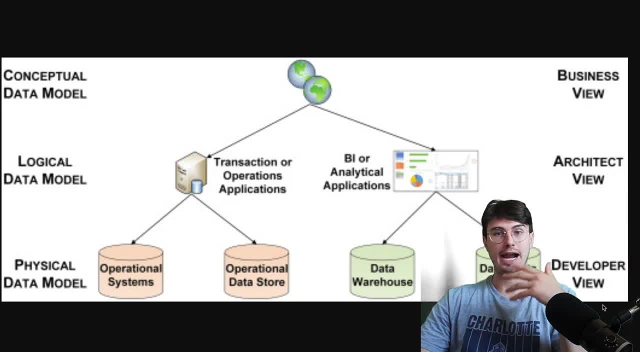 applications, whether you're, you know, a bank or an applicant. you know, and you like someone like Facebook collecting information about their users, understanding how the interface is collected, stored and then used. So it helps you. you know so some of the benefits of this. you know you. 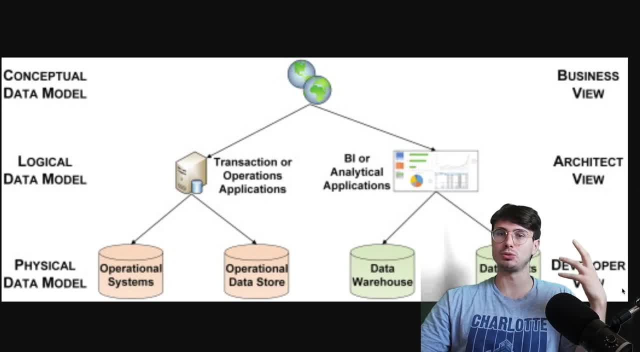 have database design helps you to you know, identify the right data structure, understand. hey, this is the type of data we're collecting, these are the types of things we want to do with it, And so data modeling allows you to define the relationship. 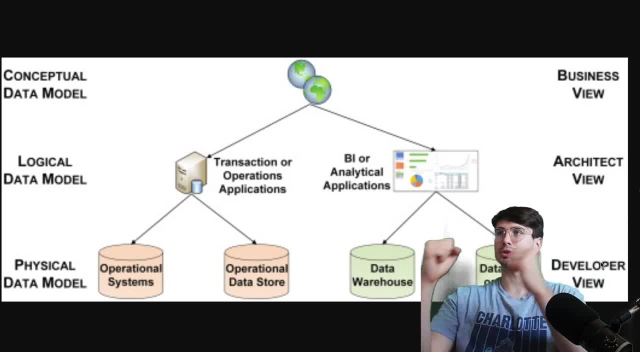 say, hey, how are we bringing it from that raw data into usable data that then can be easily used by our developers? So that's kind of the architect's job, figuring that out. And then this ensures, you know, obviously, data integrity and accuracy. make sure that if we're doing things, 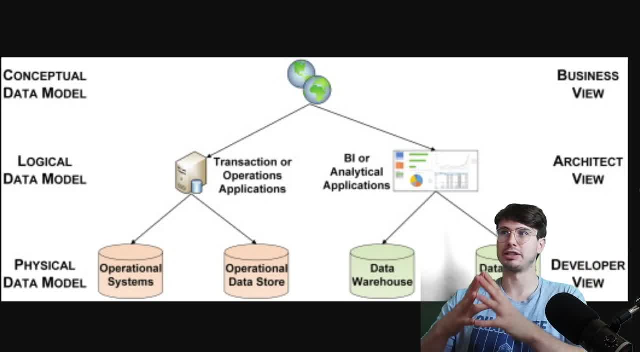 like AI ML, that we're actually training our model on relevant data and not just completely screwing it up and setting ourselves up for failure by making inaccurate predictions. And you know, kind of hand in glove with this, you have data analysis. 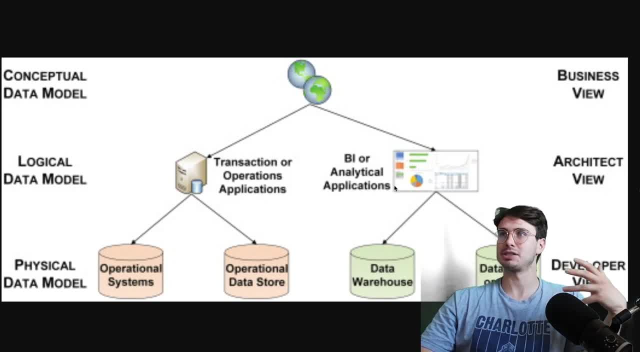 you have, you know, bringing your data from its backend databases into BI or analytical applications, for you know people to actually gain insights from all the data that you're painstakingly modeling all day. You know it doesn't mean anything if no one's actually using. 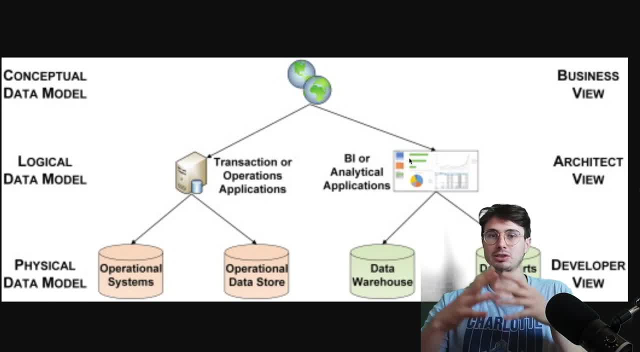 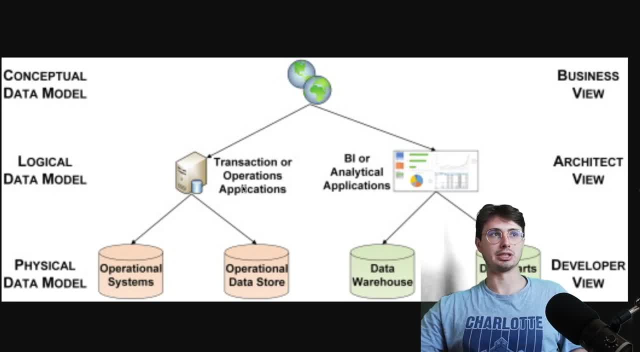 how is our data going to be used in applications So you can look at, you know, your transaction operation applications. management of that understanding you know how you're storing your transactional information- to kind of use the example here- and ensures that the data that 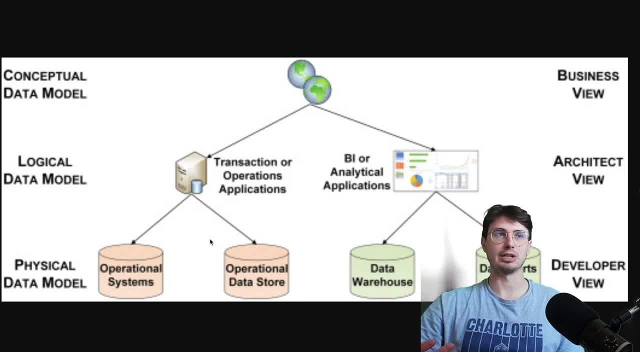 you're handling from your applications is accurate and consistent, So you're not storing inaccurate data around. you know your purchasing patterns, so that you're then, you know, not misled about what your customers are actually buying, And then also at kind of a more, I guess, boring level. 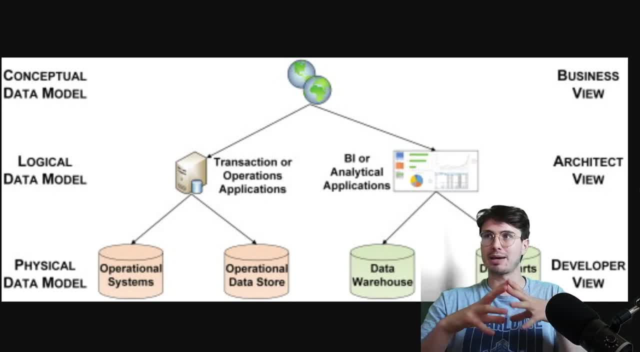 it provides data governance. So gives you a common vocabulary, clear understanding of: hey, this is where all of our data is stored. by having that mapping out of, you know, hey, this is where all of our data is, what types of data we're storing, where it's stored, what you know, security. 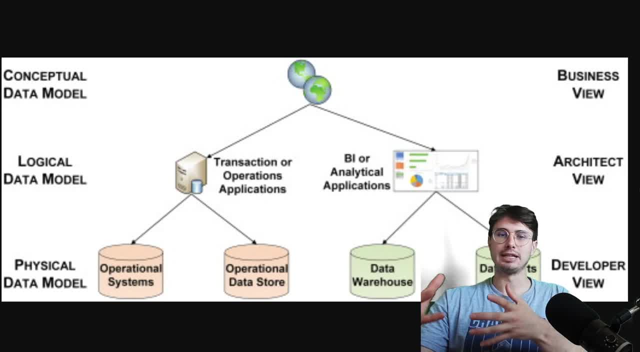 measures are taken on that data And that can also help you in compliance with any kind of standards and regulations And obviously for any kind of financial institution, that's really crucial- or any GDP compliant or GDPR compliant organization as well, Because the Europeans 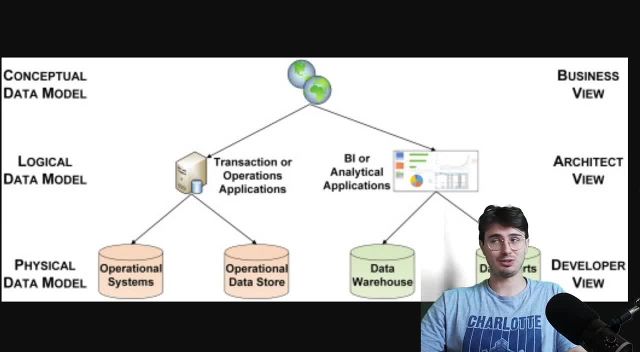 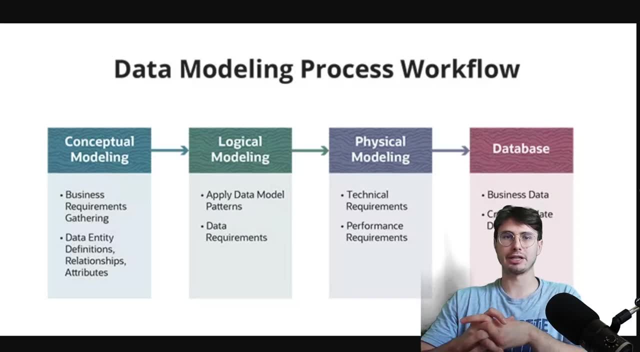 love, love protecting personal data, which is awesome. And so to kind of like guide you through a typical workflow you're going to be going through when you're establishing data modeling- Number one, conceptual modeling, which is just really getting the high level insight of what 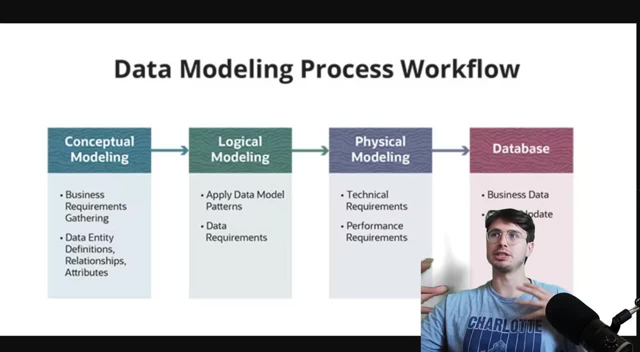 is the data we're working with. What do we want to do with it? What do we need to store? What can we prune, maybe as we ingest it? What do our end business, user, stakeholders, so the executives, need to see in their analysis or in their report? And then, of course, we're going to be looking at 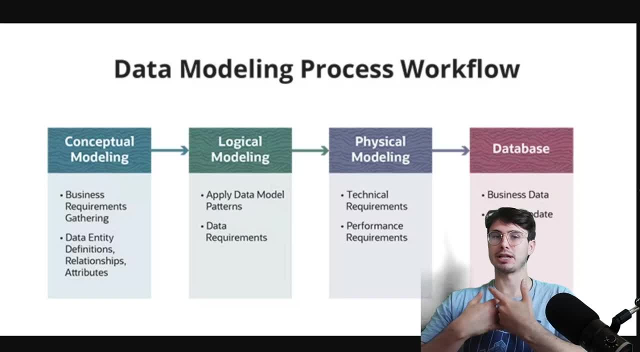 reports, making sure that that data is stored properly, collected properly and defining how it can be used for our analytics engineers, or just analytics data scientists, to actually produce those reports easily. That would mean them needing to constantly come to us and ask us: oh actually. 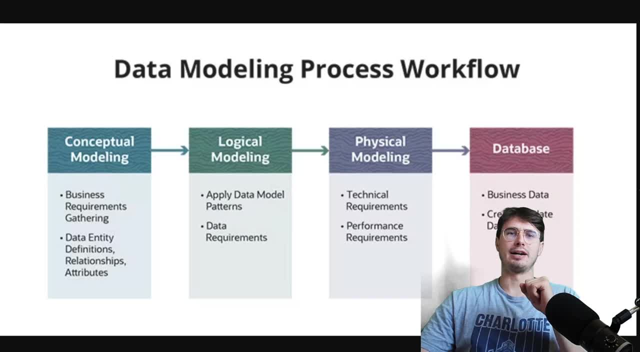 we need to change this and do that and blah, blah, blah, blah, blah blah. So this also involves conceptual data modeling. So you know, as I said, high level representation based on those stakeholder requirements. not really very technical. 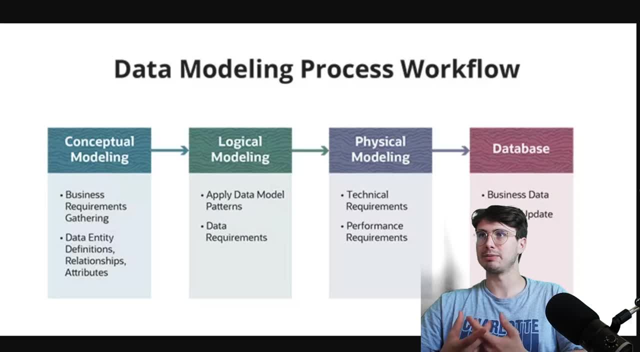 More something that you'll want to present to you know someone that doesn't really understand databases but understands what that data needs to be used for. Then, after you've gotten all that set up, you'll then want to go into the logical data modeling section and develop a really detailed 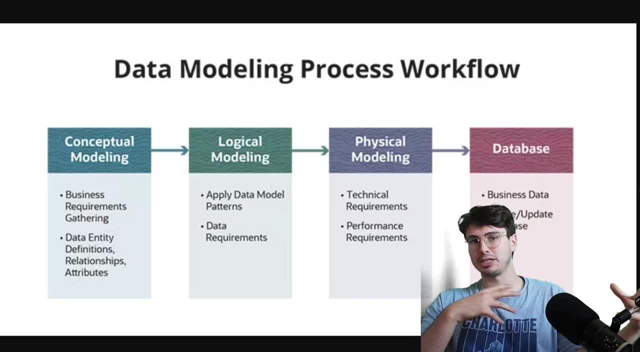 technical model that includes your attributes, primary keys, foreign keys, relationships between different tables, and you know, just really map it all out in actual technical detail And also understand. you know, hey, what is the kind of data we're ingesting, What are the attributes of? 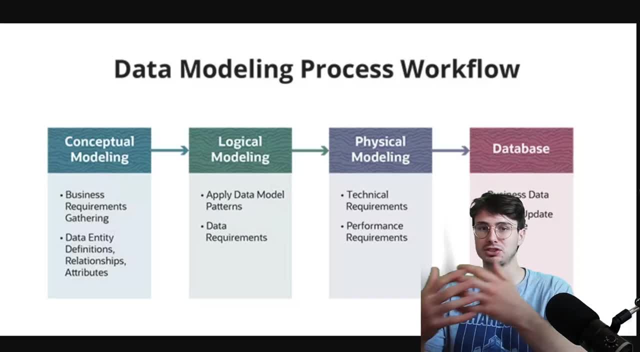 that data And really just set that up. And then you know, we're going to be looking at a lot of different things. So you know, if you're going to be building your database, you're going to have to actually set up your database. you're going to have to set yourself up for success when you actually 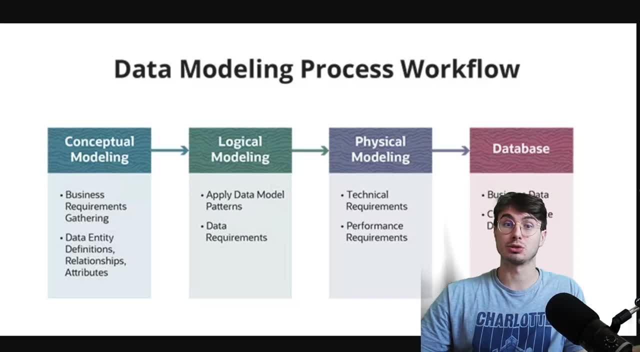 start ingesting it And when you're going to start ingesting it and set up, actually build your database is in the physical modeling stage. So you're not actually going to build a database from scratch. it's not hardware, But you are going to be creating your database schema based on that. 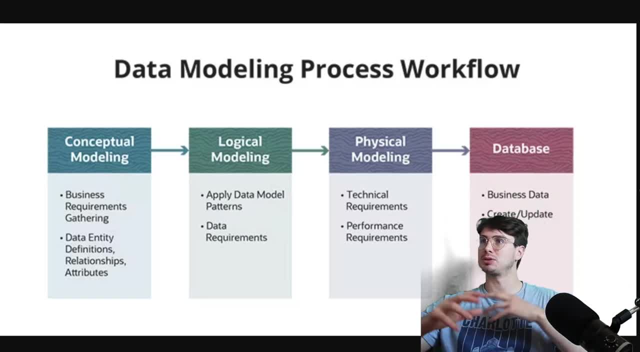 logical model. So designing, you know, schema and all the different layers between those databases and then optimize, you know, for performance, indexing, partitioning, maybe sharding different databases. whatever you need to do there, do it before you actually start ingesting the data. So 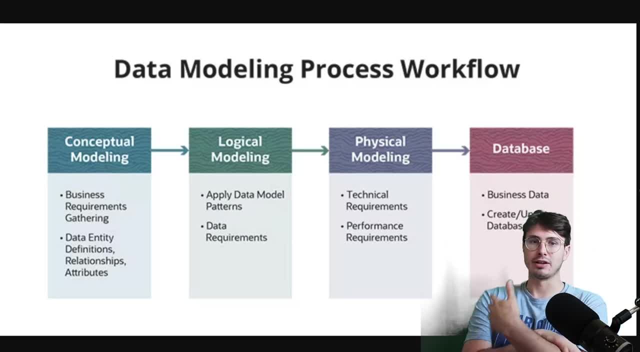 you don't have to move around data After, And then finally you'll actually create the database and start uploading your business data, But then the kind of hidden fifth step is maintenance. So you're going to have to deal with things like data change, capture over time, And maybe, you know, maybe sometimes, hey, executive. 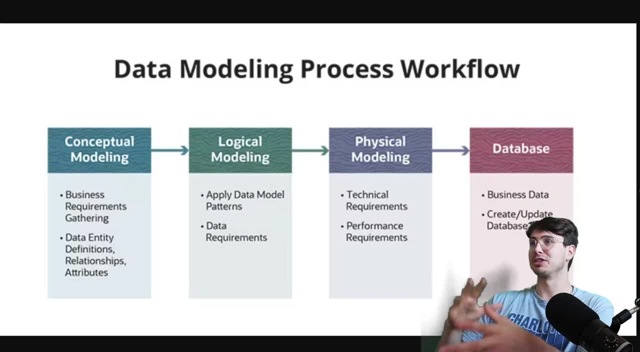 says, I actually need to get this pie graph up. you'll have to go there and change your data model to actually reflect that. So you're going to need to make sure you document everything, make sure everything is human, readable, legible, that you can go back and make any changes easily. rather, 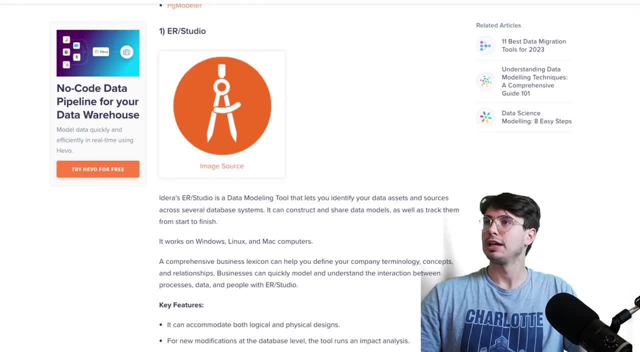 than having to, you know, comb through spaghetti code and tactical debt. And so, because data modeling, you know it's, obviously you're not going to take your data model and just like paste it into a database, you're going to just use a data modeling tool is really to kind of visualize. 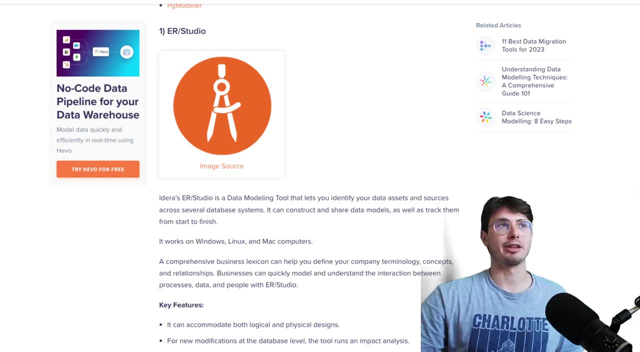 So any design tool that you're already using you can probably use for data modeling, But there are also some dedicated tools for this. So the most popular one is er studio, And this actually lets you plug into your databases and kind of identify them, identify. you know relationships between 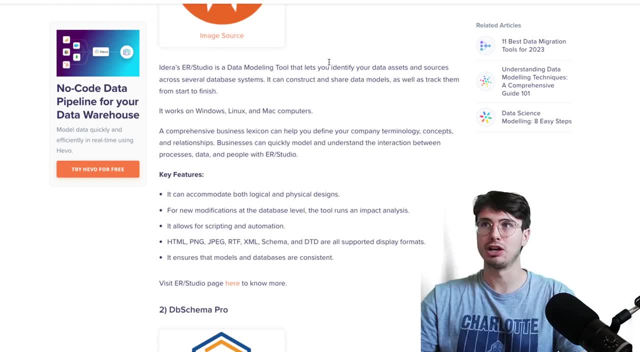 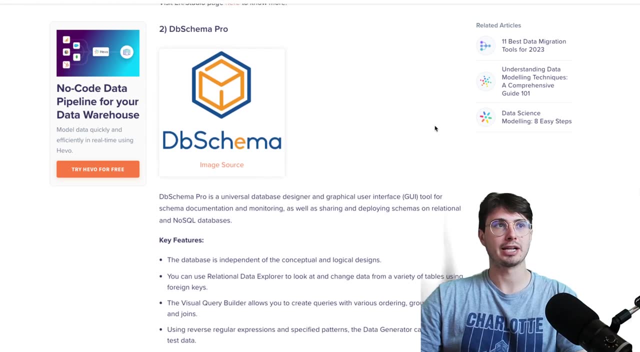 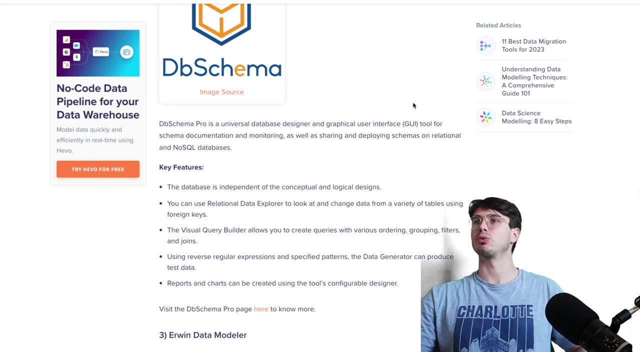 your data. It also allows you to, you know, design yourself within your data modeling tool. You also have DB schema. So schema documentation, monitoring, scaring schemas, unrelationable and no SQL databases. you can quickly, you know, copy and paste complex schemas for if you want to replicate a database from. 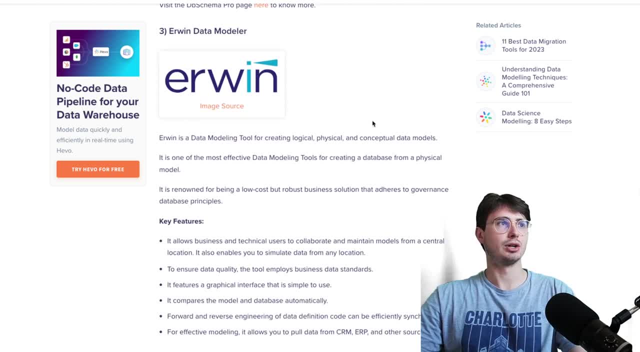 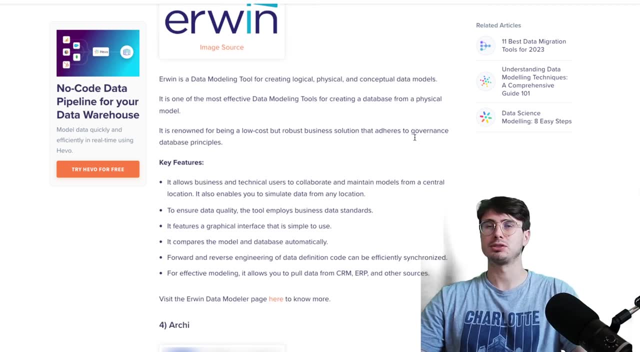 one to another. You also have Erwin data modeling, So this is creating a database from physical model and actually does allow you to interpret. you know what your specifications were and create a database. So remove some of the steps and you still have to write out all the different steps in your physical 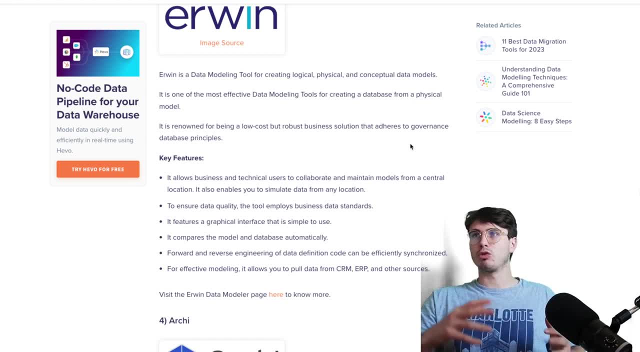 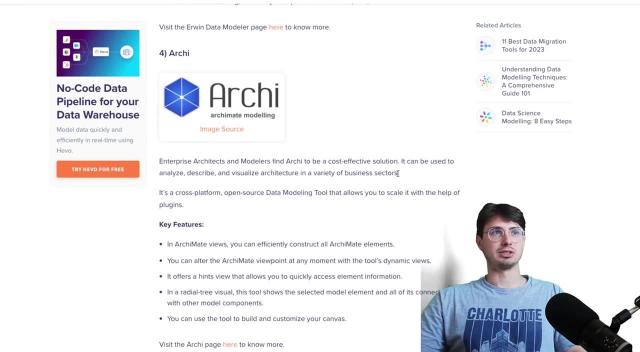 model. But instead of just kind of doing the double work, you can, if you do it right, format in order initially, it'll automatically apply it and build that database. If it's compatible, of course, you'll save Archie, which is, you know, cheap solution- allows you to just visualize, inscribe. 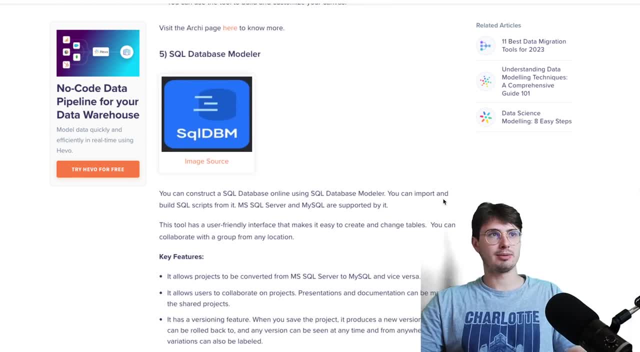 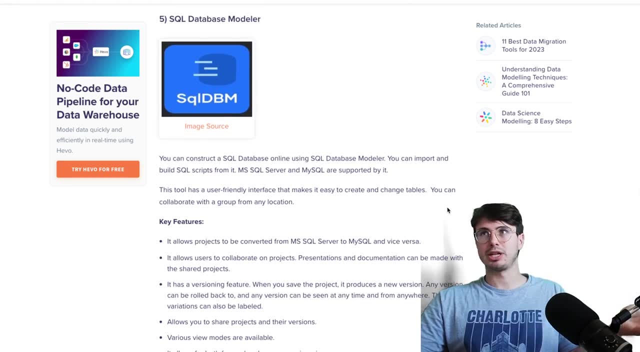 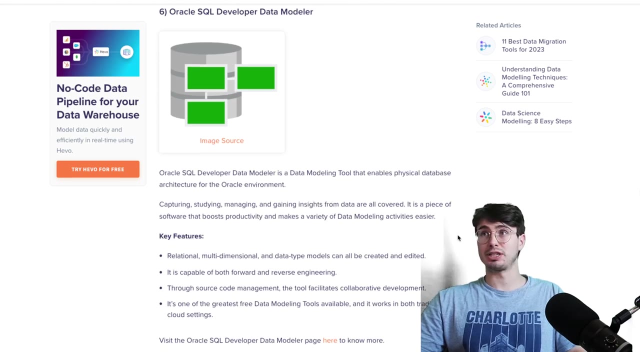 architecture, So just pure visualization tool, SQL database modeler- And this is again. you can build a model within, see it within SQL database modeler and then use it to build a corresponding SQL database. You also have Oracle SQL data modeler, if you're still using Oracle databases, And then IBM infosphere data architect. 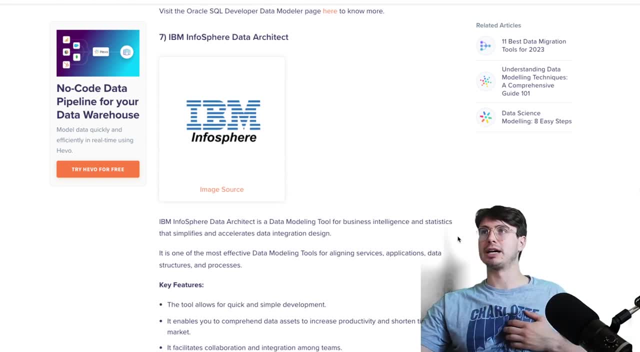 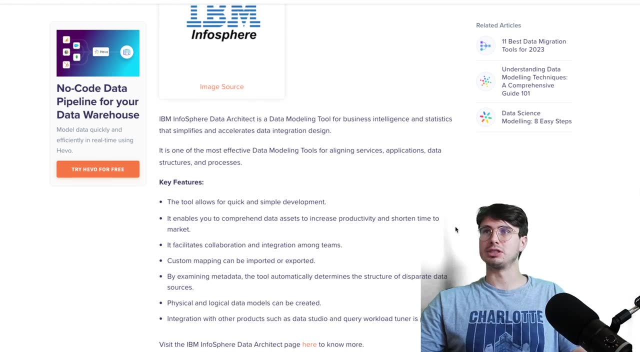 which is really built for you know business intelligence, simple and statistics. So really good for you know. if you're not super, you know data engineering, focus and you're just want to say, Hey, how are we adjusting data and then bringing them into our analytics platforms, my SQL workbench? So 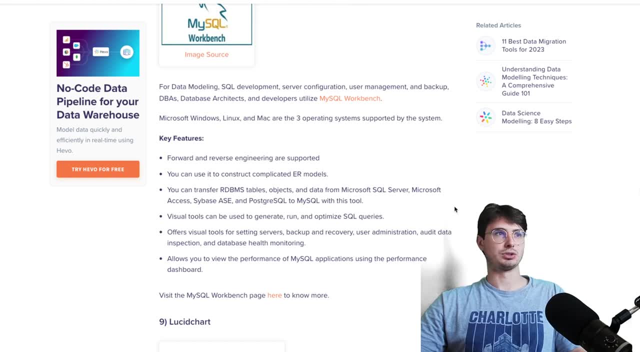 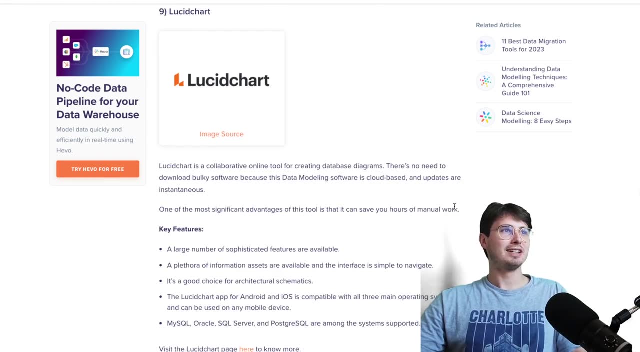 just, you know nice open source figure. you know allows you to construct models For my sequel. however, I hate working with my SQL So I'm not even gonna touch that Lucidchart. This is, you're just nice collaborative online tools. If you're working with many different people, you have a large 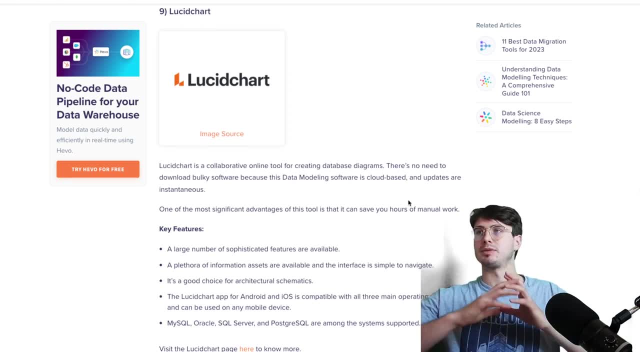 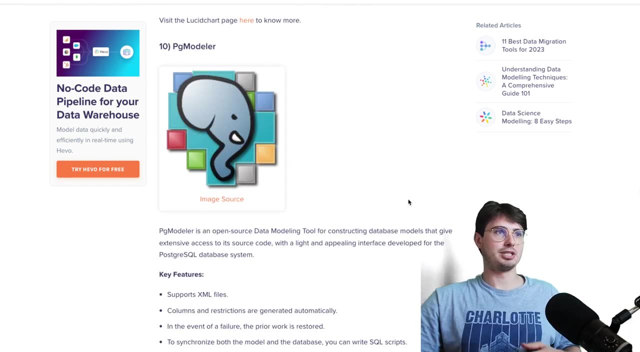 team. there's a lot of different features that you can use within Lucidchart And you know it's all cloud based, So you guys can collaborate on your models together. And then you also have PG modeler, which is open- other open source tools. So I've got to work the open source tools in. 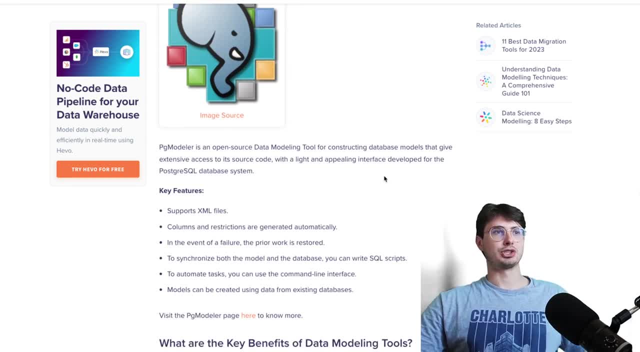 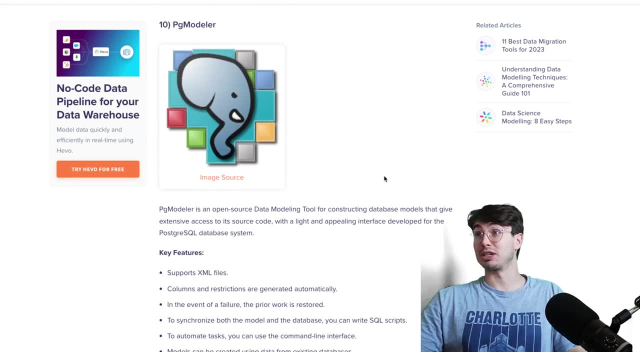 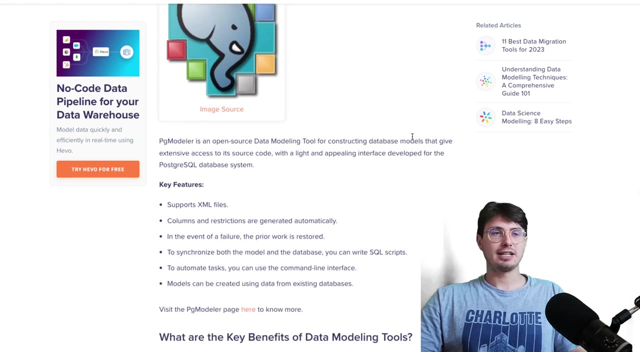 That has complete access to its source code And it's just, you know, super easy way to write a model for pd or for post, pg, SQL, PostgreSQL databases, And yeah, so that's kind of all I have for you today. I just really wanted to go into. 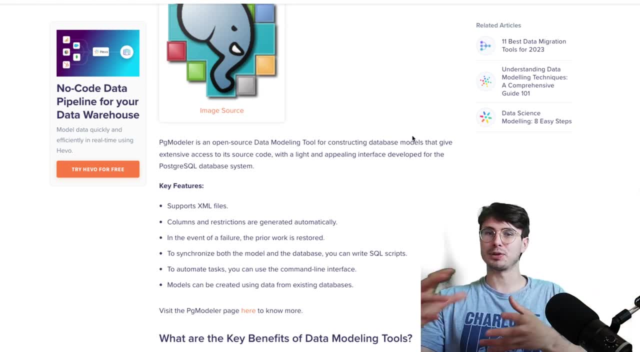 kind of everything around data modeling per that viewer request and just talk about, because data modeling is really indispensable in the modern world. It's the bedrock upon all of your data. all of you know. even data quality is built on top of data models. allows you to do actual